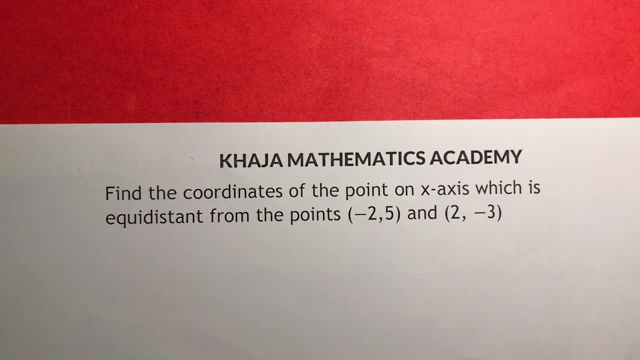 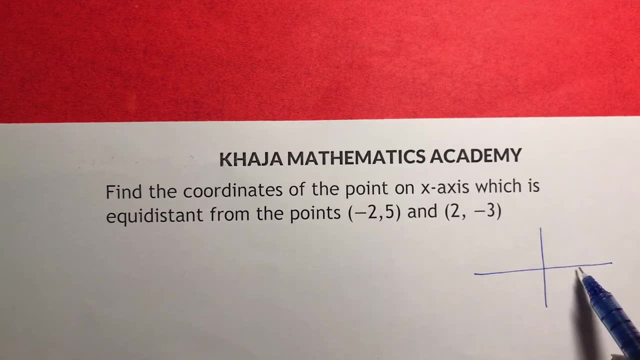 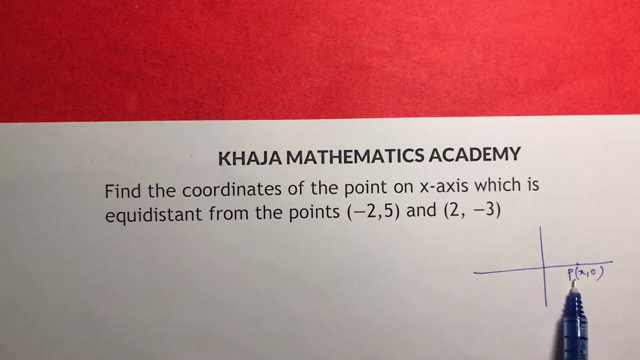 Find the coordinates of the point on x-axis. So we need to find the point on x-axis. So on x-axis, if we consider any point, that will be like x 0. So here I'll take: the point on x-axis is x 0.. On y-axis it will be 0, y if we take on y-axis, but here it is x-axis, so the point is x 0. This point is at equal distance from the point on x-axis. 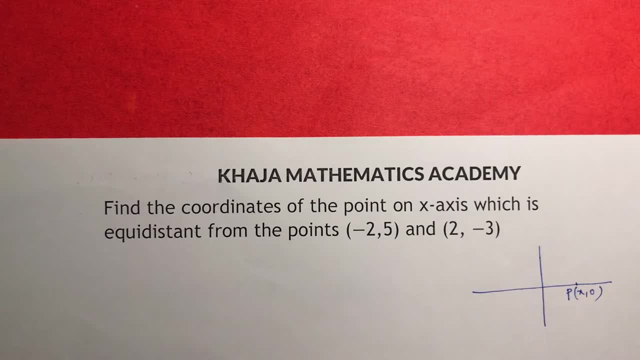 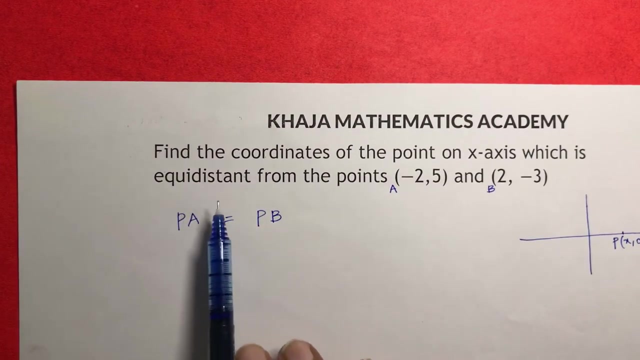 So these two points minus 2, 5, 2, minus 3.. So they gave P-A distance will be equal to P-B distance. This point I'll consider it as A, this one I'll consider it as B. Now they said equidistant. It is nothing but equal distance. P-A distance is equal to P-B distance. 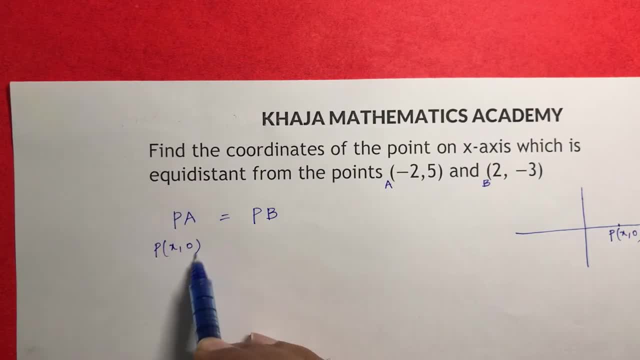 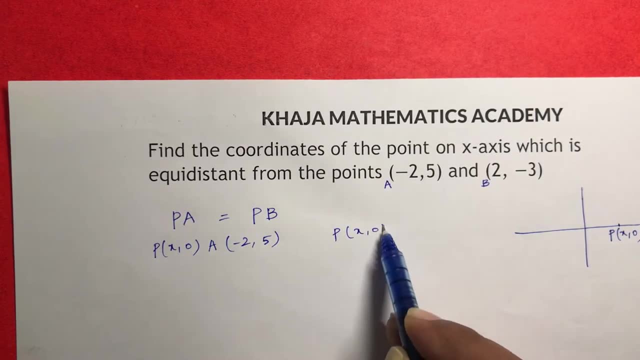 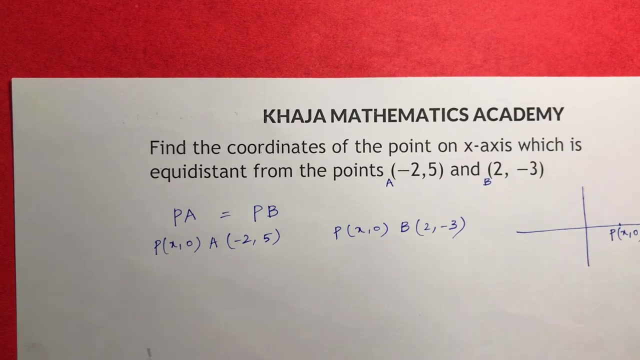 Now P is x: 0 because the point on x-axis A is minus 2, 5, 2, minus 3.. 2 comma 5, P. X comma 0, B. 2 comma minus 3. so now, if we'll find the distance, distance, 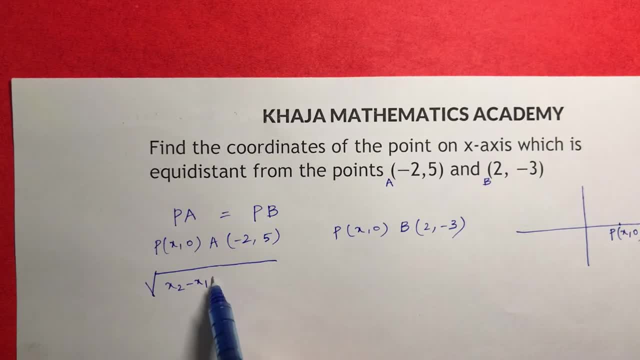 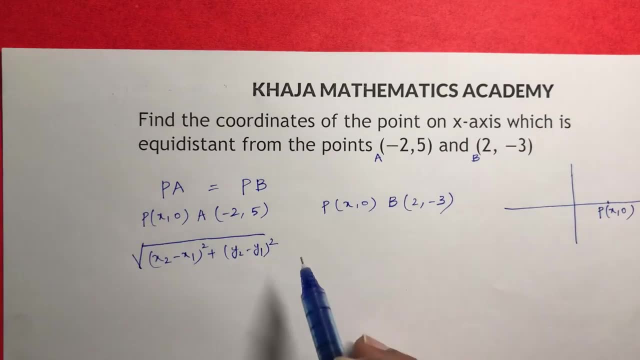 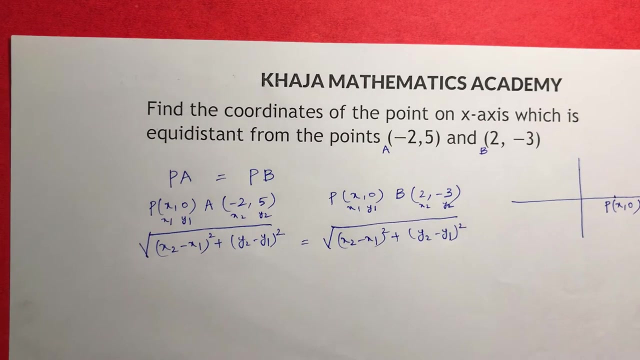 formula is under root: X 2 minus X 1 whole square plus y 2 minus y 1 whole square equals distance formula: X 2 minus X 1 whole square plus y 2 minus y 1 whole square. here you can consider the X 1, Y 1, X 2, Y 2, X 1, Y 1, X 2, Y 2. so now, if we'll 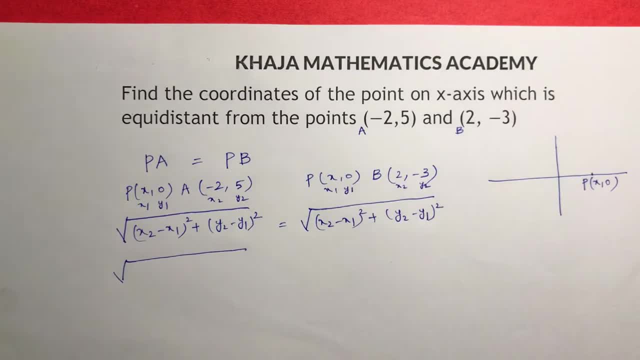 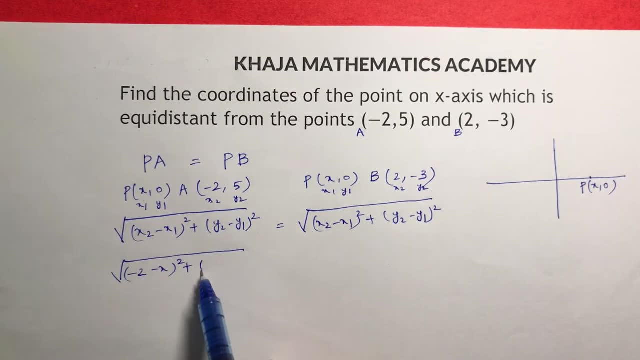 substitute the values: X: 2 is minus 2 minus X, 2 minus y 1 whole square. so you can substitute the value X: 2 is minus 2 minus X, 2 is x minus 2 minus x whole square plus 5 minus 0 whole square. now here under root: 2 minus x. 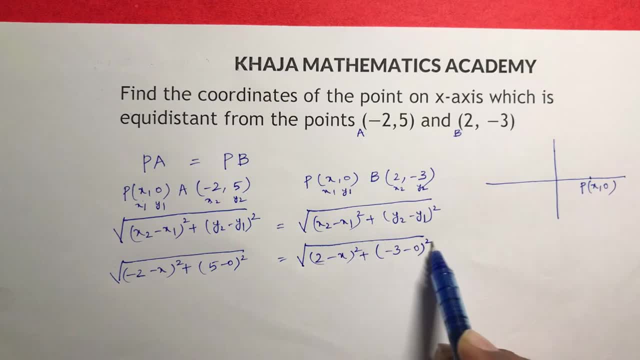 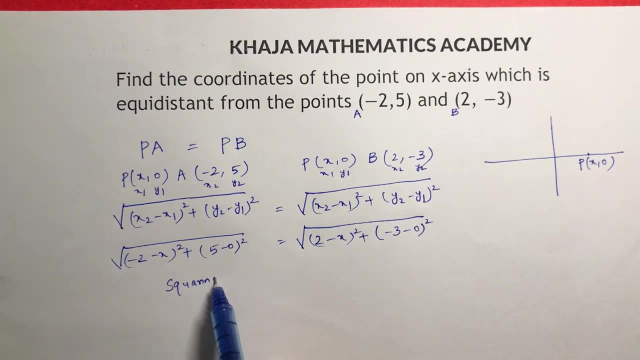 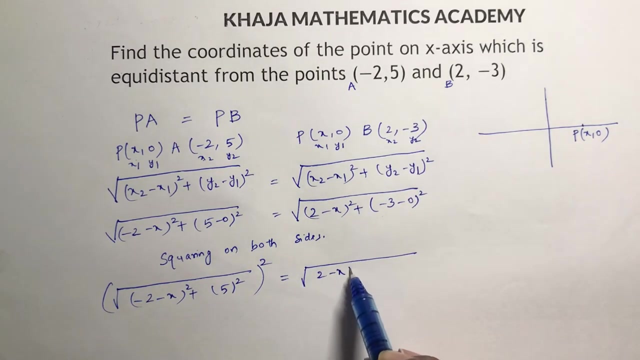 whole square minus 3 minus 0 whole square. now we have root on both the sides, so we'll do squaring on both sides, squaring on both sides. so it will be root minus 2 minus x whole square plus 5 square whole square equals root 2 minus x whole square plus minus 3 whole square and for this it is. 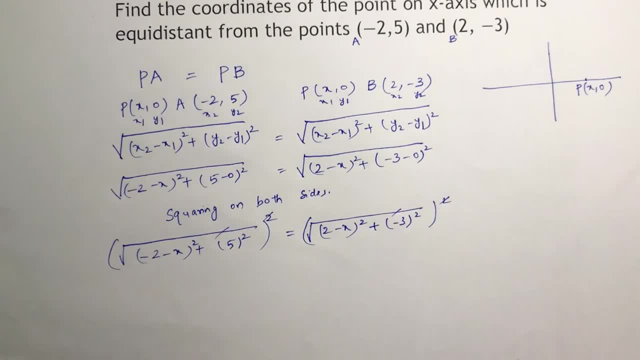 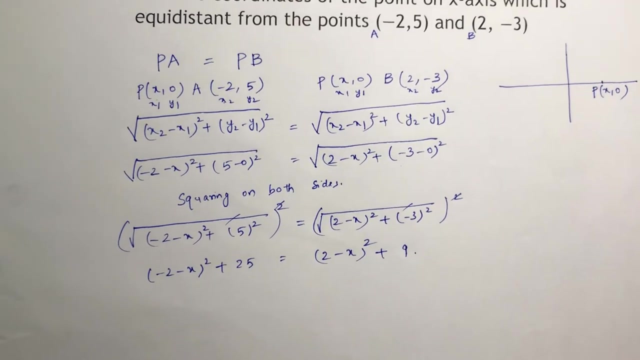 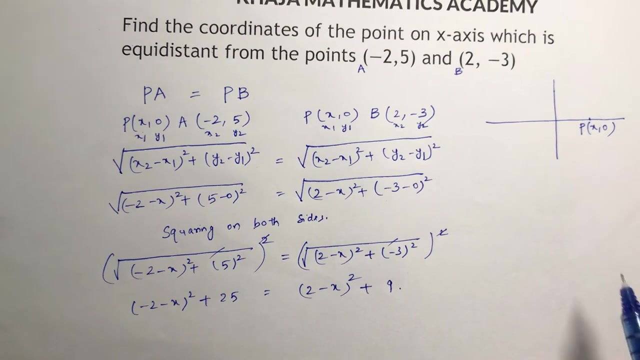 whole square square and root will get cancelled. so now what is left? minus 2 minus x whole square plus 25 equals 2 minus x whole square plus 9. now here: this is in the form of a plus b whole square. when both are minus, it is in the form of a plus b whole square. if you want to do minus 2 minus x whole square, 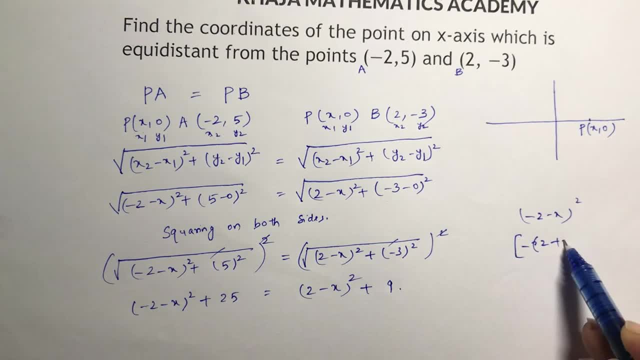 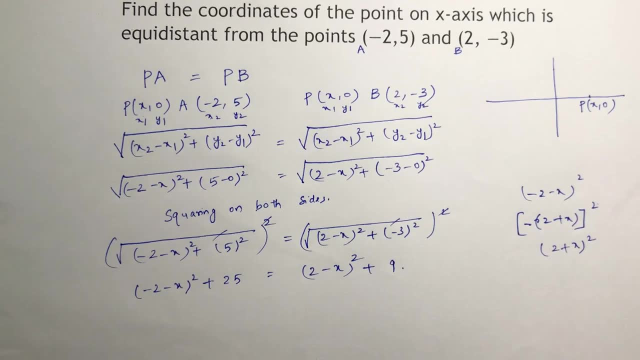 now in this: if you will take common, so 2 plus X whole square, so minus whole square is plus only, so it will be overall 2 plus X whole square. so a square plus 2 a, B plus B square plus 25, here 2, 2 B and here B, here a minus B whole square. so a square minus 2 a B. 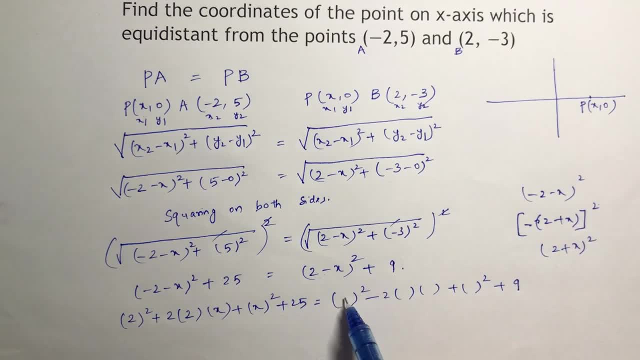 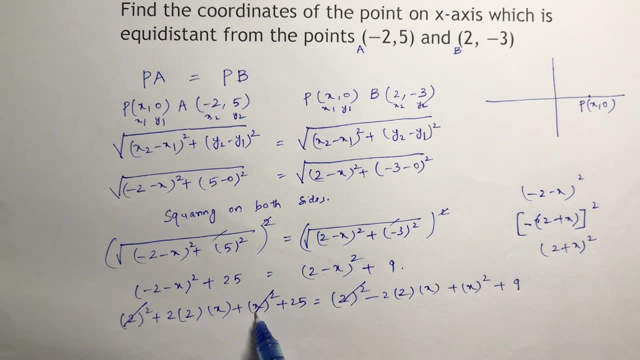 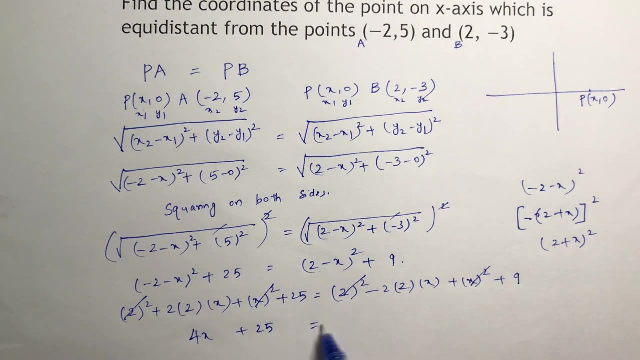 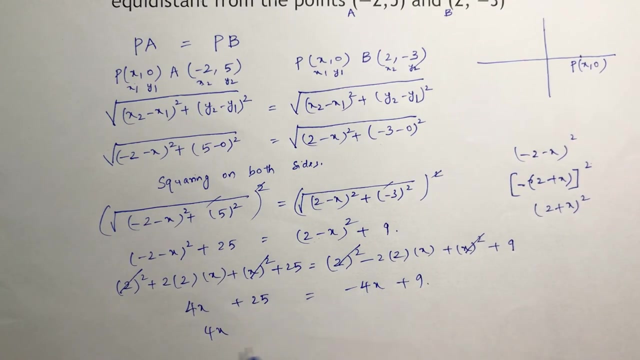 plus B square plus 9 in place of a, we have 2, so 2 here in place of B X. so now here, 2 square and 2 square, X square and X square. you can cancel. so here till like 4 X plus 25 minus 4 X plus 9, so 4 X. on transposing, if you bring this 4 X. 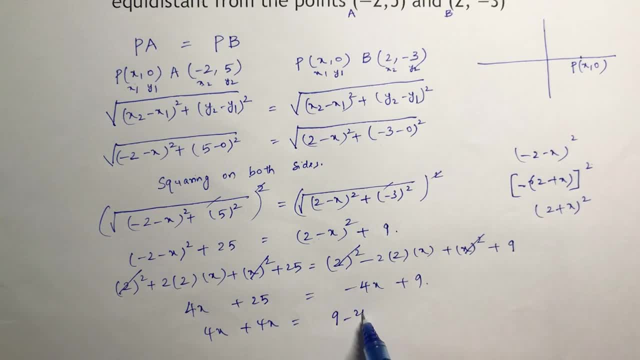 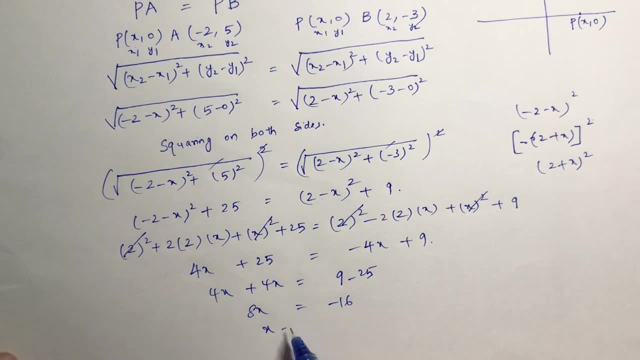 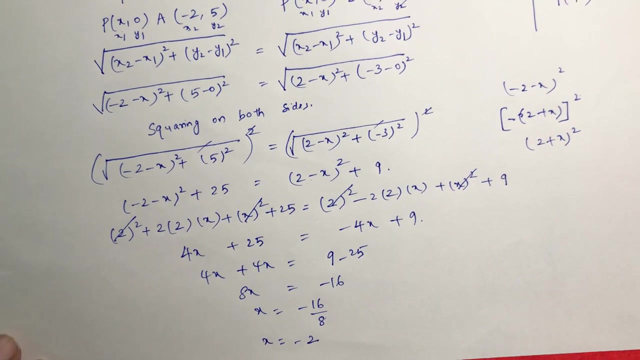 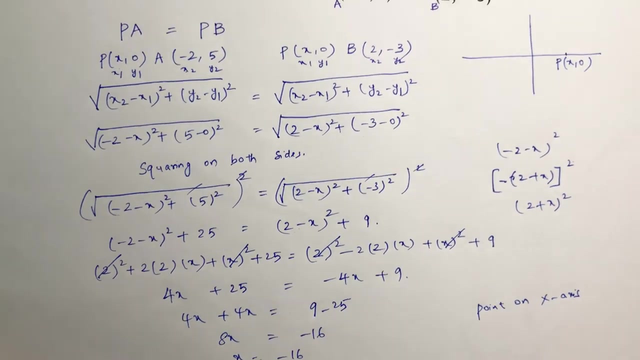 here 4 X plus 4 X is 9 minus 25. so 8 X equals minus 16, X equals minus 16. by 8 X equals minus 2. so point on X axis, which is equidistant from both a and B, is minus 2 comma 0.